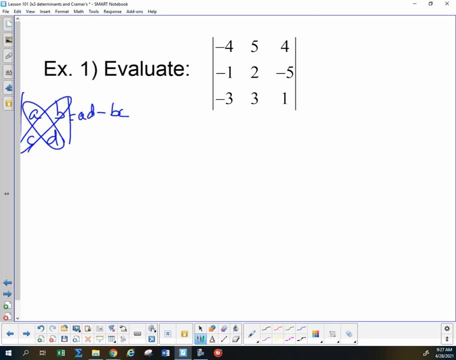 I have four numbers that I never even use. I've got four numbers in that matrix that aren't even on a diagonal, So we're going to adapt our method just a little bit. First thing that you need to do is to copy it down with the bars, and then we're going to recopy. 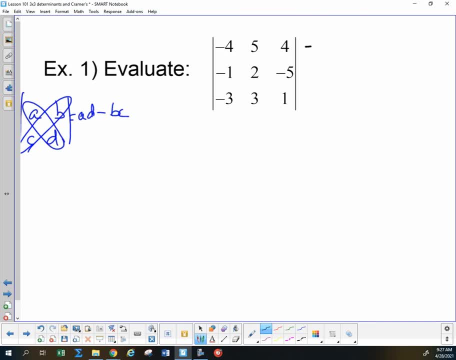 the first two columns, So the negative 4,, negative 1,, negative 3, and the 5,, 2, and the 1.. We are still going to take diagonals that go. that should have been a positive 3.. Thank. 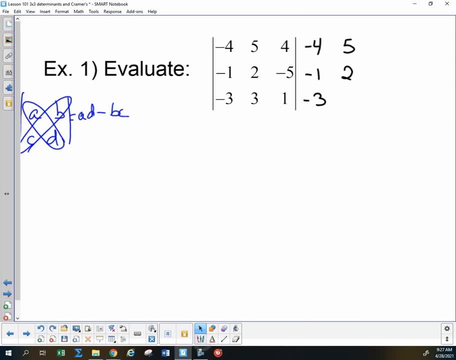 you for that correction before we went any farther. So 5,, 2,, 3.. Do I have that right now? Okay, thank you for that catch. So now what we are going to do is we are going to look at our diagonals that go upper left to lower right, And I now have a three-by-three. 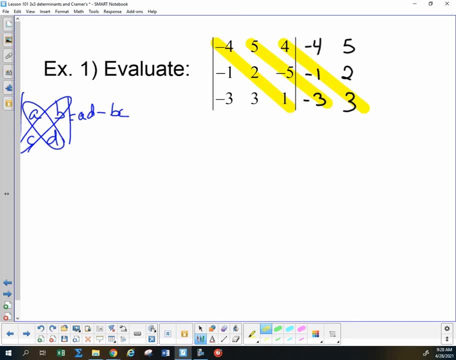 matrix. There are three diagonals about 1 and 1.. And this one is a positive. So I will probably cut all of the diagonals and just write down the positive 5,, the negative 1, and the 1. These diagrams. here I'm going to be going to actually write down the negative 4.. So 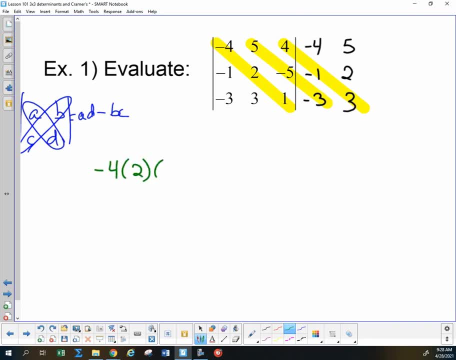 I'm going to do what I did before. I'm going to multiply all along each of those diagonals and you would probably normally not write down negative 4 times 2 times 1.. But you would just say that is what Negative 8.. And check my work here as I go. Don't let me make any. 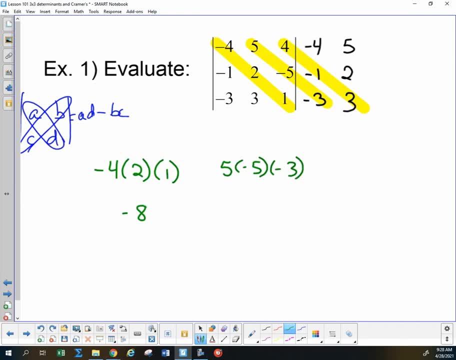 5 times negative, 5 times negative: 3, so 2 negatives are a positive, 25 times 3 is a positive: 75. And 4 times negative, 1 times positive: 3, so that is negative 12.. So those are all the ones that go from top left to bottom right. 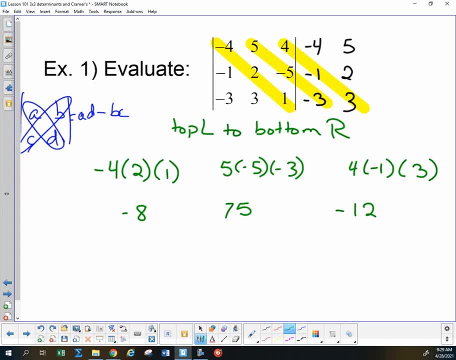 And when we did them on a 2 by 2,, top left to bottom right was always the positive one. So if they're still going that same direction, they are still going to all be positive. so I'm going to put pluses between each of those. 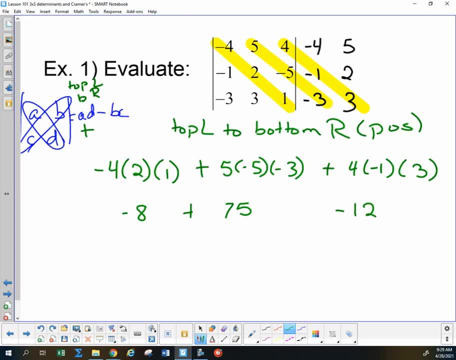 So I have negative 8 plus 75 minus 12.. Now I'm going to do 3 diagonals that go the other way. So I'm going to have these 3 diagonals, So the ones that go bottom left to top right, bottom left to top right. 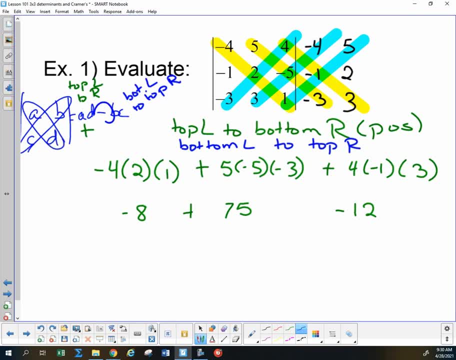 bottom left to top right And that diagonal is going to be negative 7, so it is negative 7.. So I'm going to take these 3 and divide them by 5.. Now say I want to get, I need my x and I need my y. 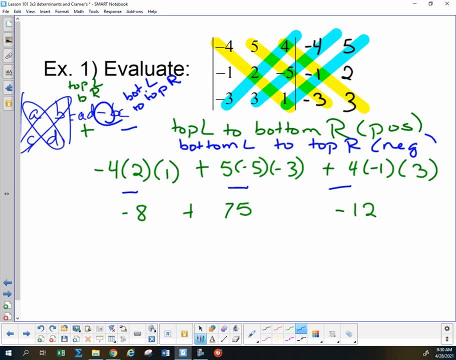 Right here I have: negative would be equal to negative. negative, 3 times negative. 3 times 4 times 4 times negative, 3 plus 4 together. so I think that means that's good. Take 3 essentials. Take 3 essentials. 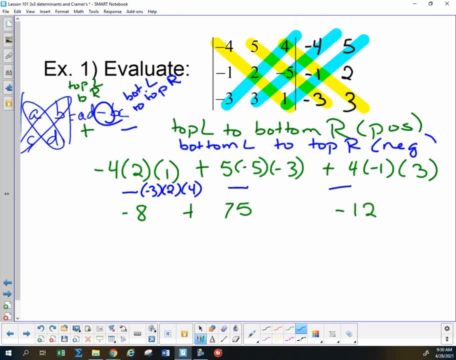 Add 3 single areas together. Add 3 until letting theutarians side stick together. Minus, minus is plus 24.. And the next one I'm going to have: minus 3 times minus 5 times minus 4.. So minus, minus, minus. 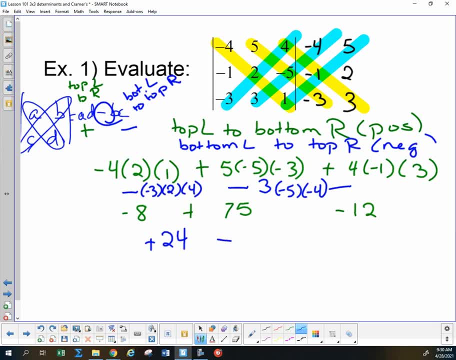 I think I've got a negative in there, And 20 times 3 is 60. And then for the last one, I've got 1 times negative, 1 times positive, 5. So negative, negative is a plus And that is a 5.. 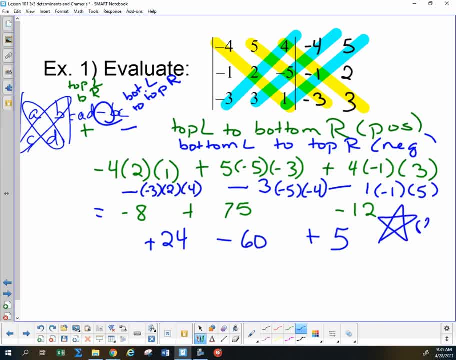 This line is required. Okay, This part is optional. In the work that I want to do, I want to see, But I want to see because you're going to make some mistakes on these And for me to help you figure out where the mistake was. 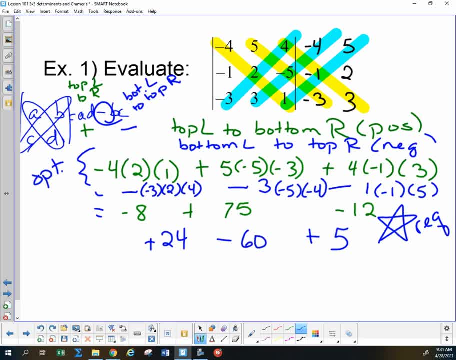 I need to know how did you get the answer that you came up with? So then, if we combine those, let's see what do we have? 99 plus 5.. So I think I have 104 from my positive ones And minus 80 from my negative ones. 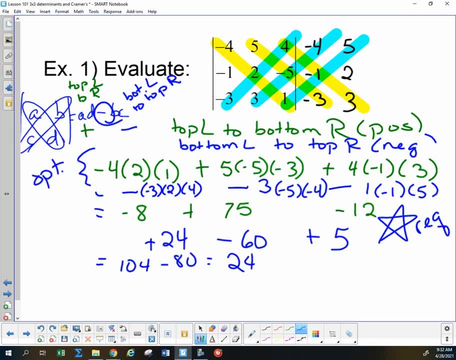 So I'm going to have a positive 24 and I do that right, So that determinant would be positive 24.. And now notice that I did use all nine of my original numbers. I don't have this negative 1 in the original matrix actually shaded, but I used it. 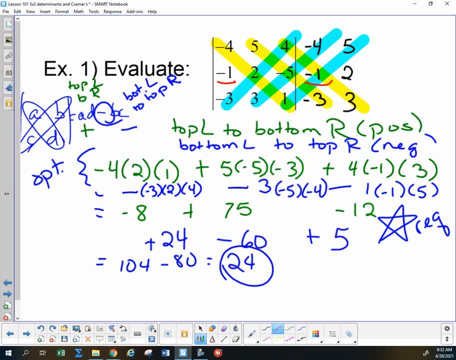 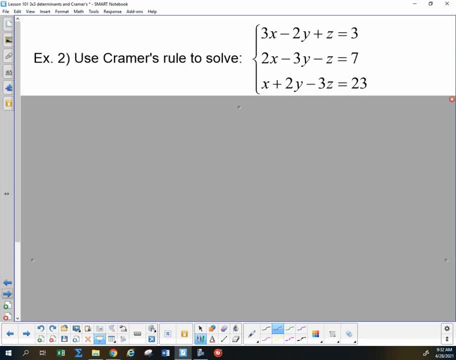 But I used it when I repeated it over here. Okay, let's keep going If we want to use Cramer's rule to solve it. Now, remember, with Cramer's rule, we needed to end up with and we just did a 2 by 2.. 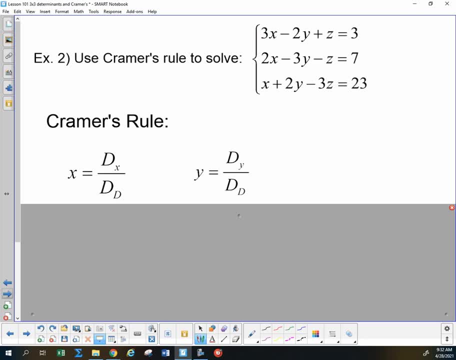 We found the determinant matrix. Then we changed the x coefficients to the constants and we found dx And we changed the whole thing. We changed the y coefficients to the constants and we found dy. And then we did dx over dd was our x coordinate of our solution. 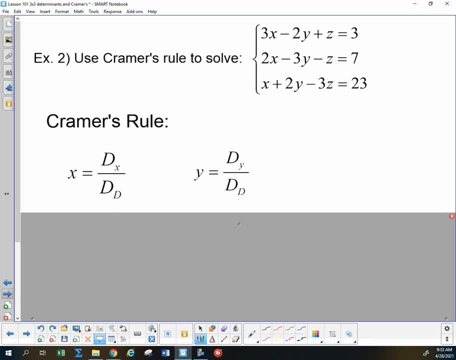 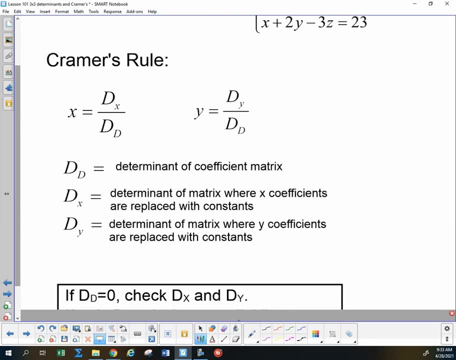 And dy over dd was the y coordinate of our solution. Okay, what we are going to do is to get a third one: dz, And dz over dd will be The z coordinate of our final solution If any of these denominators are zero, and we had this before- 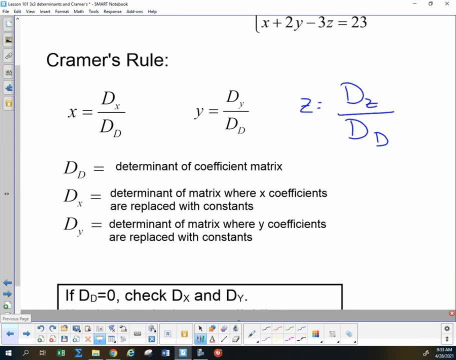 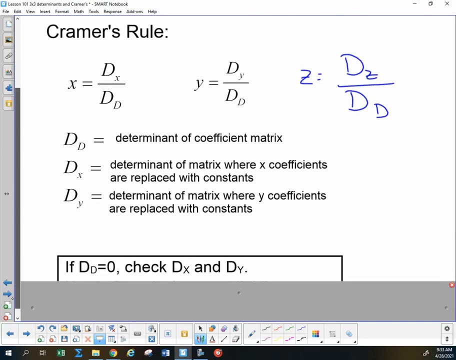 If any of the denominators are zero, that means we don't have a single point. that's our solution. We either with a 2 by 2, we either have the same line or we have parallel lines. We either had infinitely many solutions, or we had no line, or we had no solutions. 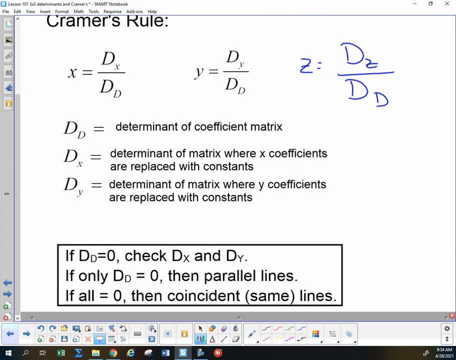 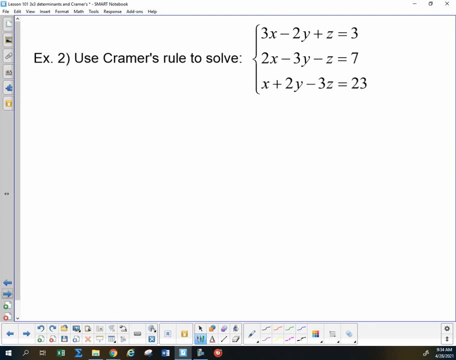 And we still. We still are going to need to do that and be a little bit different with what's going on here. But we can still have parallel lines or we could have different versions of the same line. So let's attempt to use Cramer's rule now with a 3 by 3.. 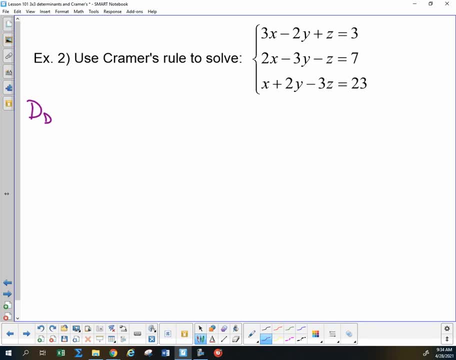 So, dd, we won't worry about the constants yet. We will just take 3, 2, 1, negative, 2, negative, 3, positive 2, positive 1, negative 1, and negative 3.. 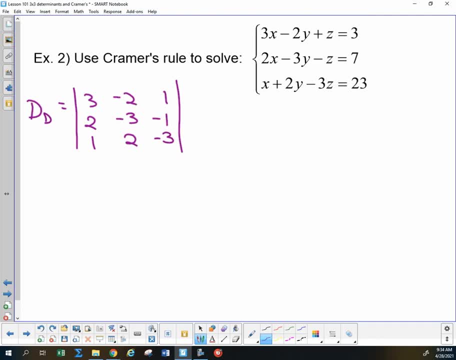 And did I get that all correct? Okay, now we recopy the two left columns, 3, 2, 1, negative, 2, negative, 3, positive, 2. And then we do all of our positive ones. So I'm going to have 3 times negative, 3 times negative, 3.. 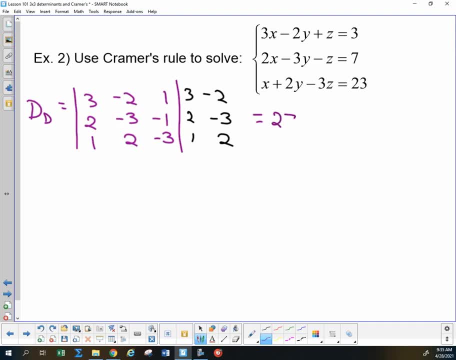 2 minus signs is a plus 27.. Then I'm going to have negative 2, negative 1, and 1.. 2 minus signs is a plus 2.. Then I'm going to take 1 times 2 times 2, those are all positives, so it's a plus. 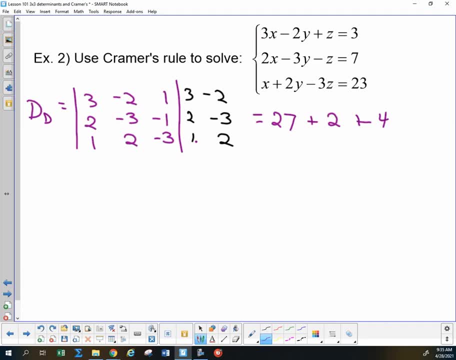 2 times 2 is 4.. Now I'm going to do the 3 in the negative direction. So I'm going to have a minus and a 1, minus 3 and a 1.. So I'm going to have two negatives which are a plus 3.. 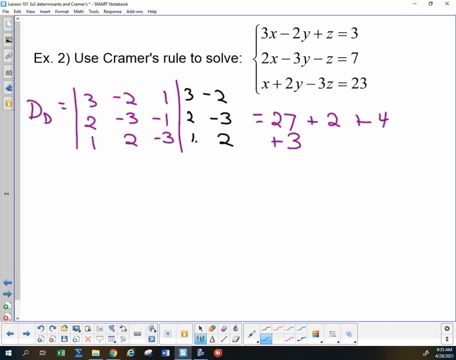 And this is also the minus direction. so I have a minus 2, minus 1 and 3, so I have 2 minus signs, So that's a plus 6. And I have a minus sign And negative 3, 2, and negative 2.. 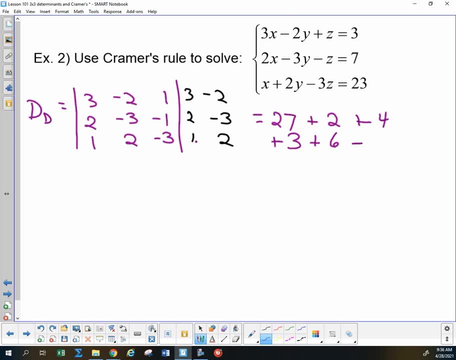 So that's 3 minus signs, So a minus 12, I think You guys are checking my work as I do that. So then if I put those together, I have 30 plus 8.. Plus 4.. 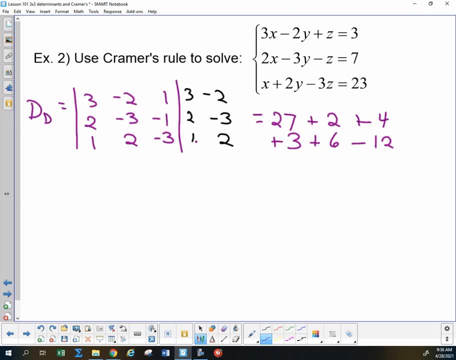 So I have 30 plus 12 minus 12.. So I believe I just have positive 30. So when I get ready to do my final answer, all of my denominators are going to be 30s, And then maybe I can reduce. 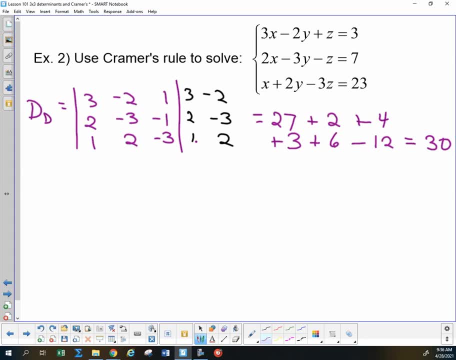 Okay, Now to do dx. I take my x coefficient. I take my x coefficient. Right where they are, I don't move them, And I replace them with the constants 3,, 7, and 23.. I keep the other columns the same. 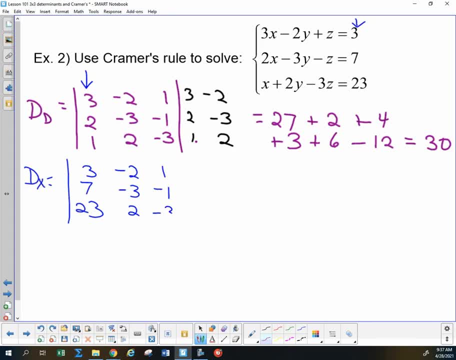 Negative 2, negative 3, 2.. 1, negative 1, and negative 3.. Once again, I need to repeat my first two columns: 1,, 2,, 3,, 4,, 5,, 6,, 7,, 8,, 9,, 10,, 11,, 12,, 13,, 14,, 15, and 18, and 19, and 20.. 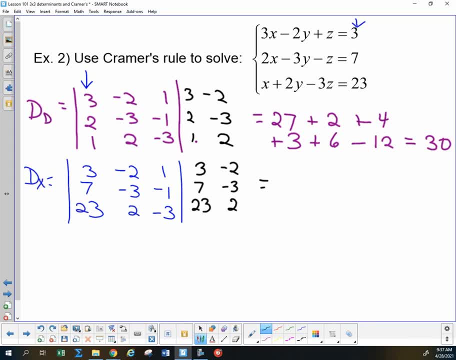 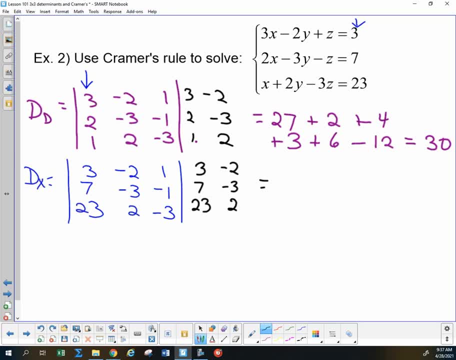 So the positive direction first: 3, negative 3, negative 3, 2, negative. So that's still a positive. So 27. Negative 2, negative, 1, 23. Two negatives is a positive. 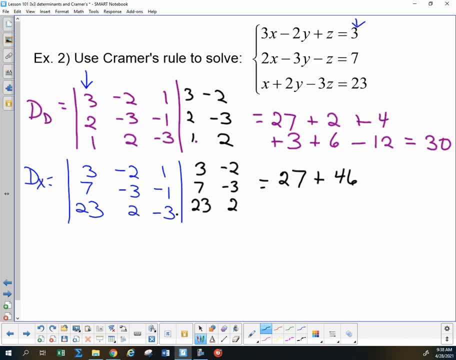 and 2 times 23 is 46, and 1,, 7, and 2 are all positive. so plus 14. now my 1 is in the negative direction, so I have an extra minus sign for each of these negative 23,, negative 3, and 1. 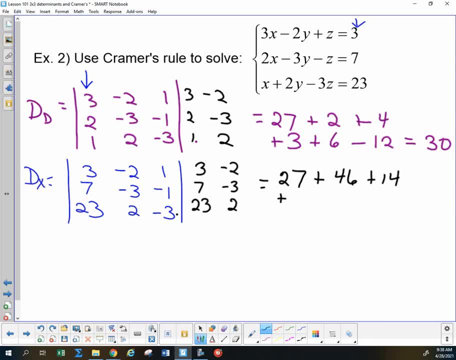 2 negatives are a positive: 69. extra negative: 2, negative 1, and 3: 2 negatives are a positive: 6 and an extra negative. negative: 3,, 7, and negative: 2: 3 negatives are a negative: 6 times 7 is 42. 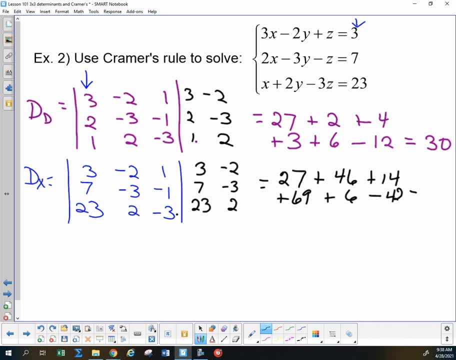 and I believe if I add those I get 120. now we need the Y numerator, which we'll call DY. here we go for the Y determinant. we're going to change these Y coefficients to the constants, so I'm going to keep the 3,, 2, and 1. 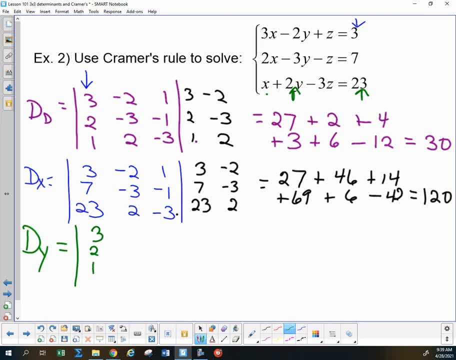 we're in front of the X's in the original problem. I'm going to change the Y's to 3,, 7,, 23 and I'm going to keep the Z's- 1, minus 1, minus 3. it pretty Broad. 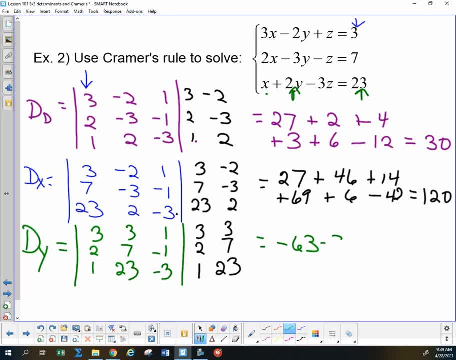 so I'm going to keep the Z's in count, so I'm going to keep the Y's in count and repeat this. repeat 3, 2, 1, 3,, 7, 23, and do my multiplying And then I have 1,, 2, and 23,. so that is plus 46.. 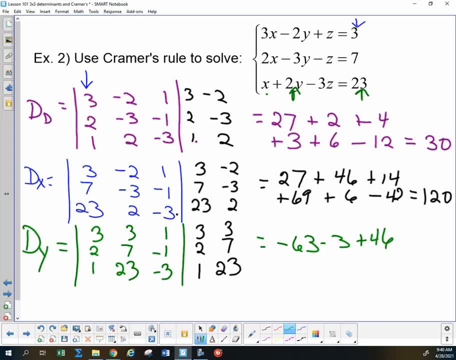 Then the 3 in the negative direction. so I have an extra minus sign with each of these, Minus 1,, 7, and 1 is minus 7.. Minus 23, negative 1, and 3 is 2 negatives. so a positive 69.. 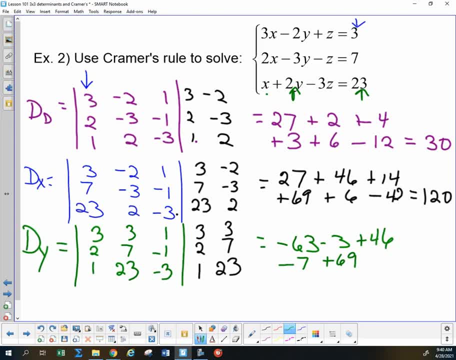 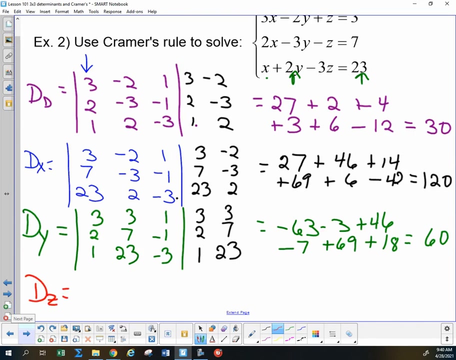 An extra minus with negative 3, 2, and 3, 2 minuses are a plus. 9 times 2 is 18, and I believe those add up to 60.. To get my Z numerator, I am going to change these Z coordinates. 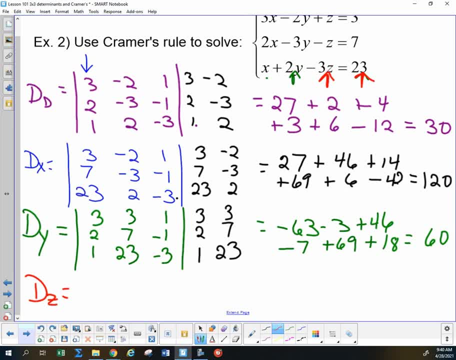 So I am going to keep the 3,, 2, 1 that I had in front of the X's and I keep the negative 2, negative 3, positive 2 that I had in front of the Y's and I change the Z's to 3,, 7, and 23.. 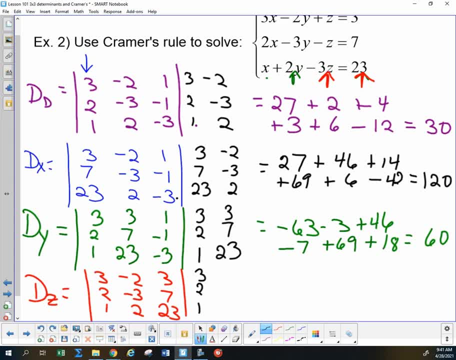 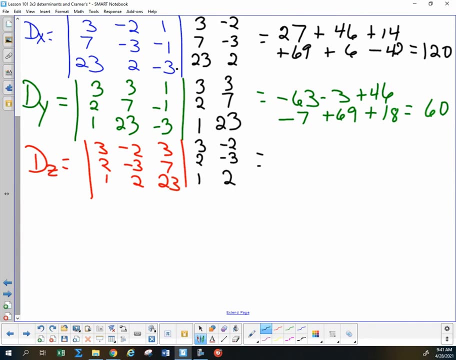 Once again, we copy the first two columns 3, 2,, 1, negative, 2, negative, 3, positive, 2, negative 2, and do my multiplying So in the positive direction: 3, negative, 3,. 23 is 1 minus sign. 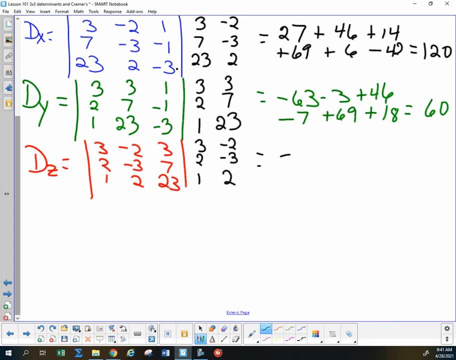 so that one is going to start with a negative 9 times 23,. 9 times 3 is 27, and 9 times 2 is 18, and 2 is 20,, so negative 207.. And then minus 2, 7, and 1 is minus 14, and 3,, 2, and 2 is plus 12.. 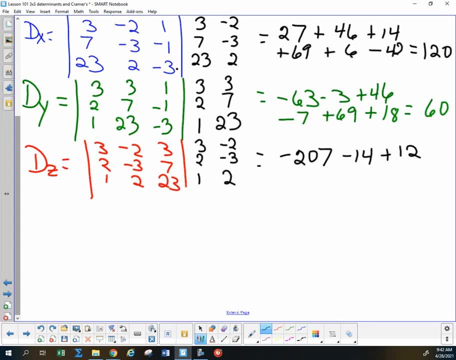 But in the negative direction. so I have an extra minus sign with each of these: minus 1, minus 3 and 3, 2 minuses are a plus 9.. An extra minus. these are all positive, so that's going to be a minus. 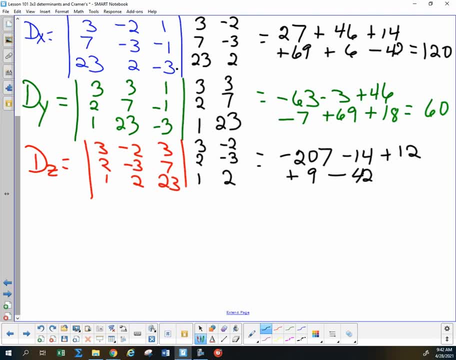 and 6 times 7 is 42.. And an extra minus with 23,, 2, and minus 2 becomes a plus and 4 times 23 is 92, and if I add those together I believe I have negative 150.. 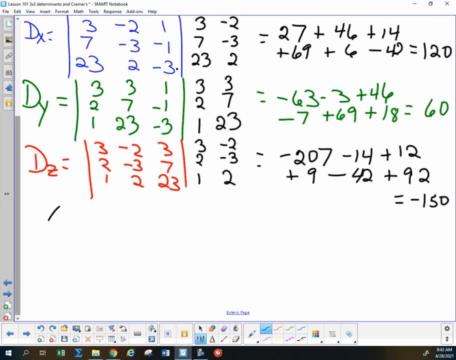 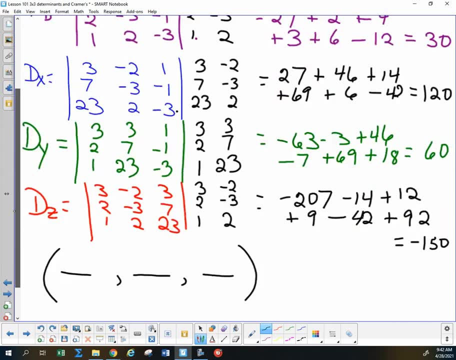 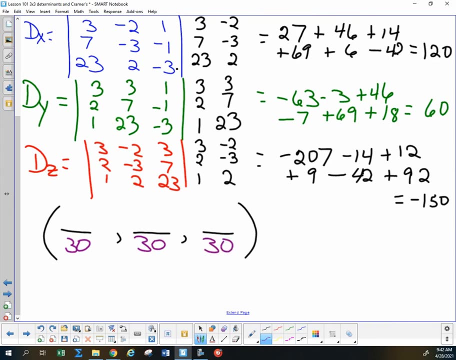 That means my final answer is going to be D D D was 30,, so all of my denominators are 30.. D X was 120,, so my X numerator is 120.. D Y was 60,, so my Y numerator is 60. 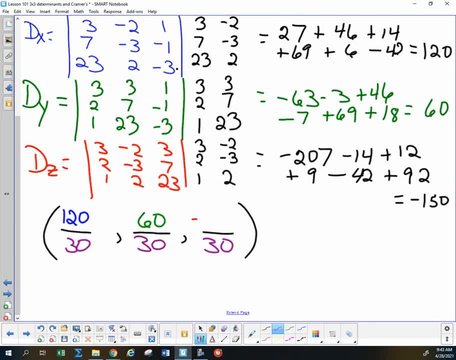 D Z is negative 150, so my Z numerator is negative 150. But all of these can be reduced for 2 and negative 5.. And there we have our answer. So just, messier, and more computations and more places to mess up. 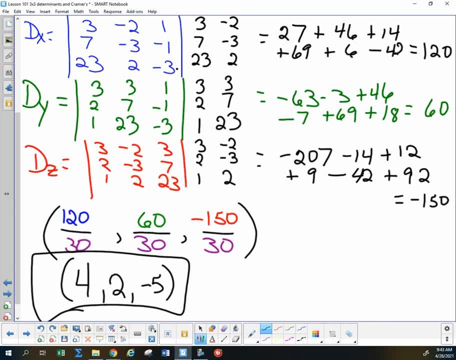 with a plus or minus sign. So you have to be careful. show me the work, Please, please, please. do it this way, For you are only writing down 4 determinants. Do not do it the book's way, for you are writing down 6 determinants. 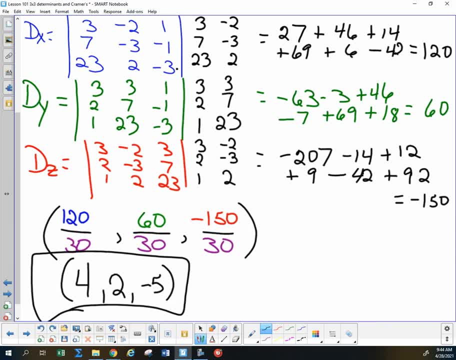 You're not going to have enough space to write determinant over determinant, Please do the D, D, D, X and so on and label which is which. It saves you time and it saves you space. Anybody with questions there? 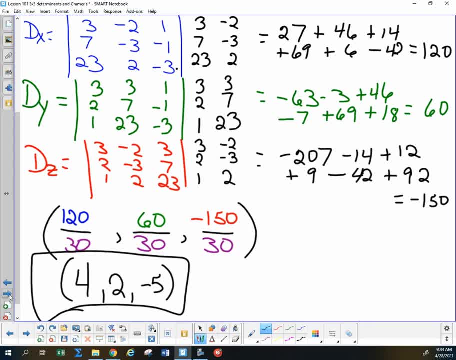 Now, fortunately, most of the time the book will say: use Kramer's rule to solve and. use Kramer's rule to solve for Y, Use Kramer's rule to solve for Z. They won't usually make you do all 3, because they get very, very messy and take a lot of time. 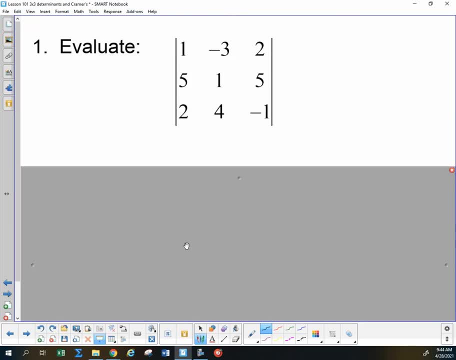 but it also means you need to read them carefully. So, you guys, just for practice, I want everybody to calculate this determinant. This is not a system to solve, so we're not getting X, Y and Z, but solve, but evaluate this and, at home, type your final number. 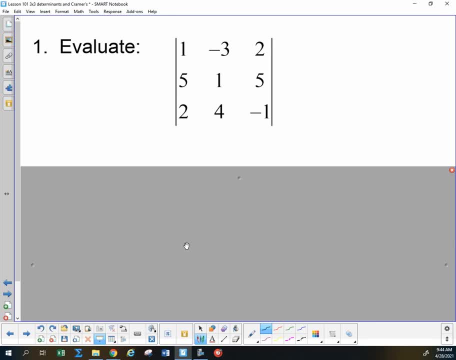 into the chat but wait to hit enter. We're going to do that in a minute, So negative 30 is majority rule here, but let's go through the steps to make sure We have negative 1, and then we have negative 30,. 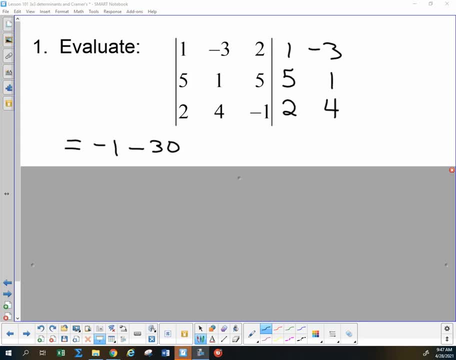 and check my work as I do this- and plus 40, and then these are all the opposites, so minus 4,, minus 20, and plus 1.. Okay, And minus 15,. did I get all of those in there, right? 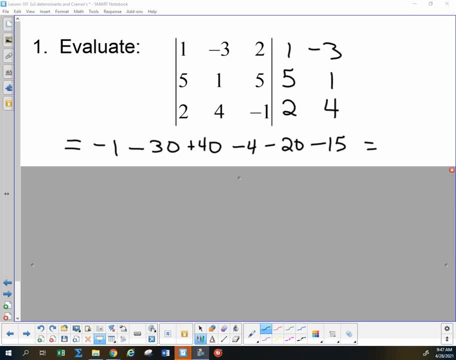 And so let's see what is that going to give me? I'm going to have minus 15,, minus 4,, minus 1, that's a minus 20.. Another minus 20 cancels with a plus 40,. so, yes, negative 30.. 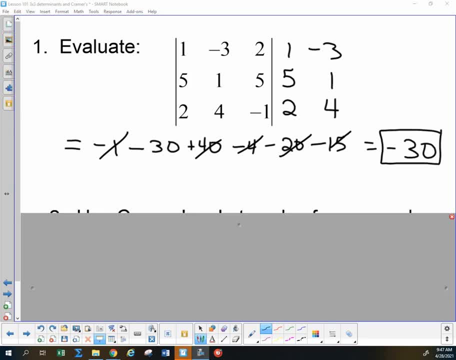 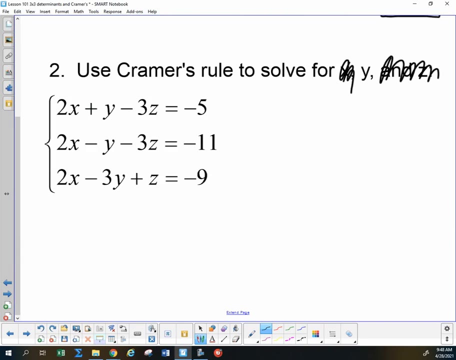 Questions there. Okay, one more of these. Use Kramer's rule. Let's just solve for Y. This way you can see it better. So which determinants are you going to need to find if you're just solving for Y, Roddy? 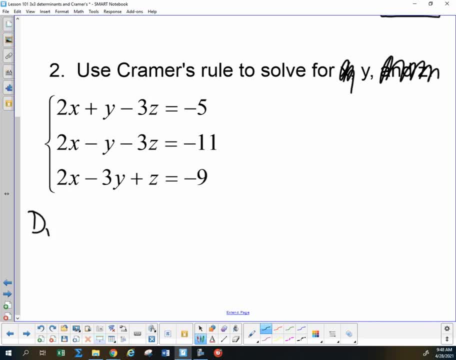 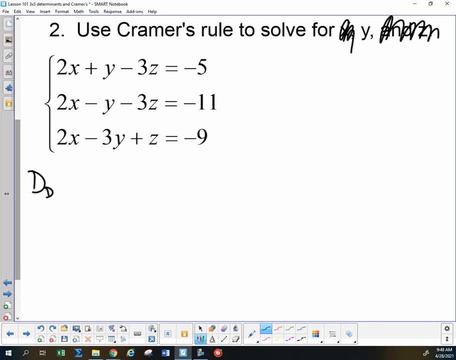 So you need to find DD and you need to find DY. It's going to be Y-y-y-y-y-y-y-y-y-y-y-y-y, And if you don't find any, then you can just write this up And that's going to be your way to get your y-y-y-y-y-y-y-y. 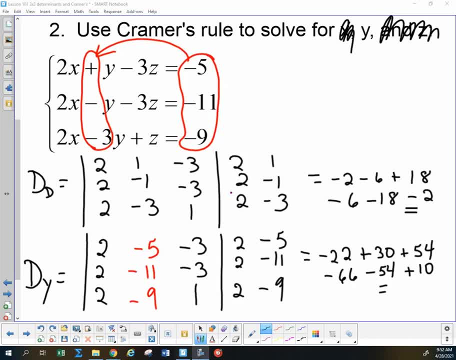 And what you're going to do is you're going to. So everybody was getting that y is 3, which is correct. I just want to talk through the work just a little bit. dd, we kept all of the original coefficients. We copied the first. 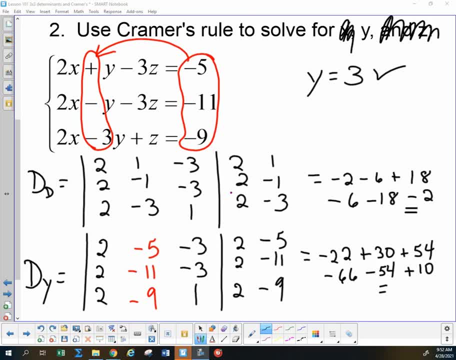 two columns and multiply all of the diagonals and I believe you got negative 16.. Is that right? for dd And then for dy, you go back to your system. you change these y coefficients that I circled in red to the constants. So your middle column is now negative. 5, negative.